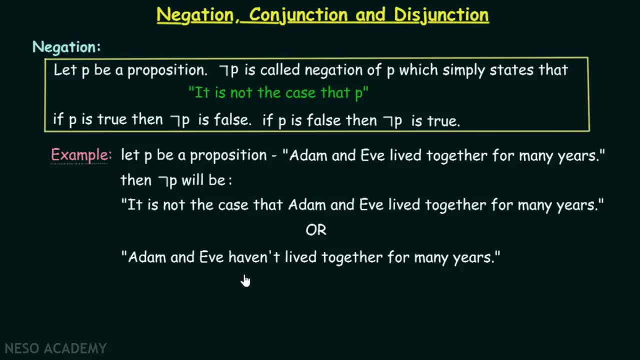 in front of the preposition You can write something else that goes with the meaning. For the sake of reference, I am providing the truth table for negation of P. When P is true, then not P means false. When P is false, not P is true. 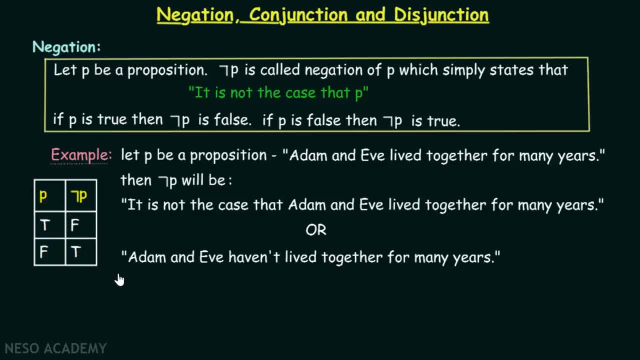 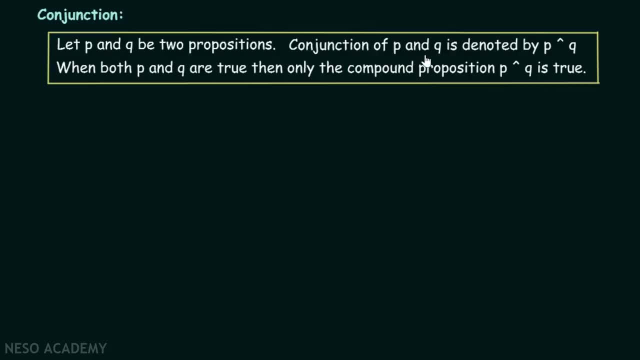 Simple. Now let's try to understand what is conjunction operator. Again, let P and Q be two propositions. Conjunction of P and Q is denoted by P and Q. This is the symbol for, and Please note down, this is the symbol. 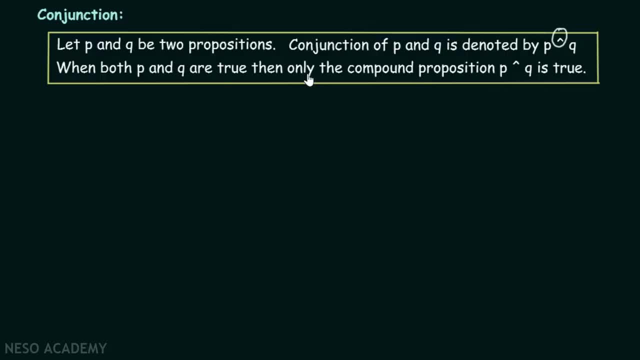 we are going to use for, and in propositional logic, When both P and Q are true, then only the compound of the preposition P and Q is true. Let's consider one example: Twelve is divisible by three, And three is a prime number. 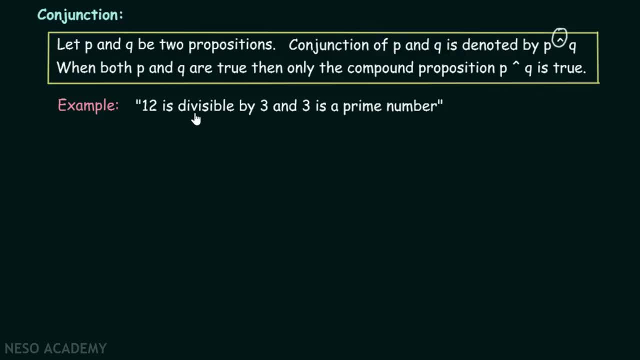 We already know that twelve is divisible by three. This is correct, And three is a prime number. We also know that this is also correct, As this proposition is true and this one is also true. therefore, true and true is equal to true. 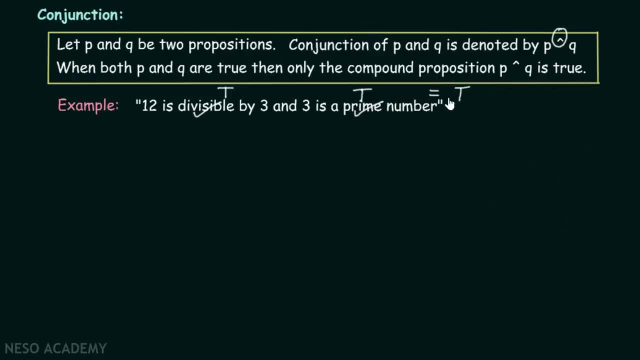 Right. For the sake of reference, I am providing the truth table here. This is the case that we are considering over here. in this example, True and true equals true. Okay, Please note down one important point: Sometimes we use but instead of and. 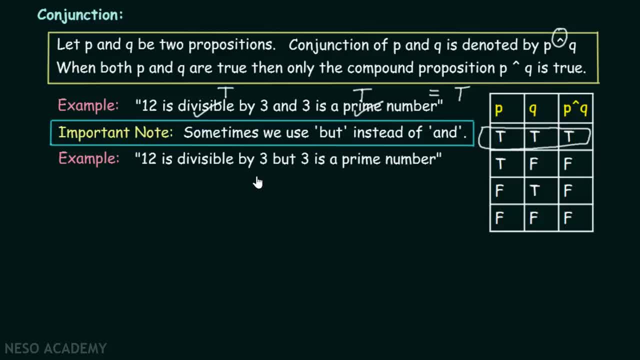 Like, for example, twelve is divisible by three, But three is a prime number Here, but is equivalent to and- Please note down this point- But and and both are same in propositional logic. When you find out, but in a statement, then it simply means and. 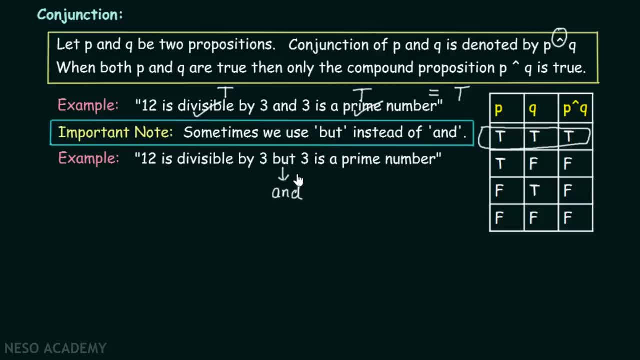 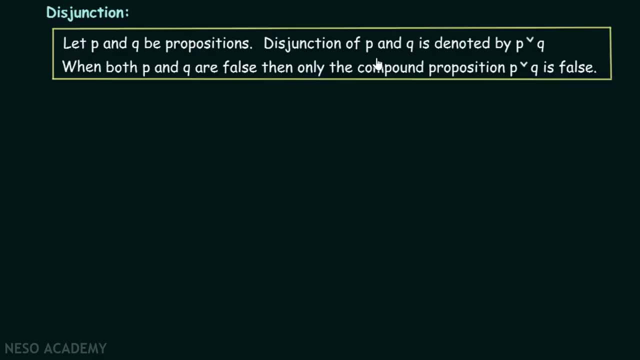 Therefore, both the propositions need to be satisfied to make this particular compound proposition satisfied. Now let's consider our third operator in the list of logical operators, That is, disjunction operator. Let P and Q be propositions. Disjunction of P and Q is denoted by P or Q.